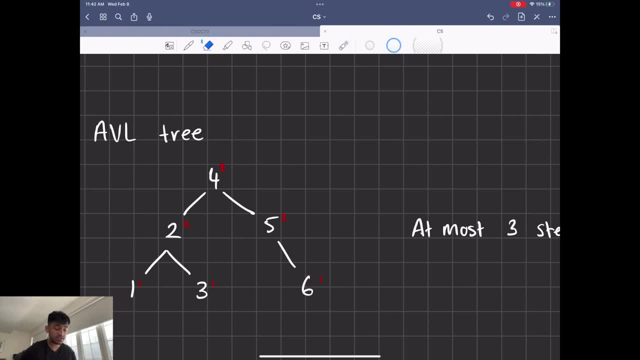 have at most 3 steps, including that first node, And you're going to see these numbers next to these nodes that represent the height of the tree at that node. So, for example, at 6, the tree is 1.. At 5, you're going to see that you only have one child, So your height is 2 now And 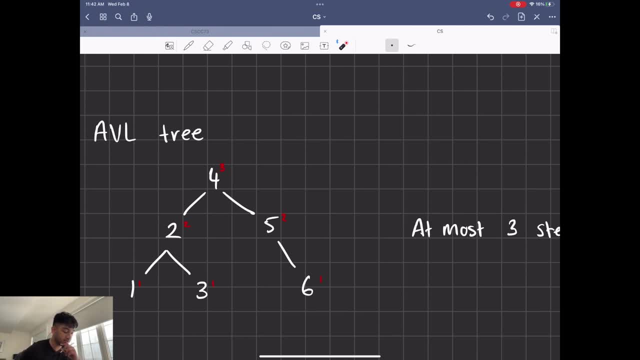 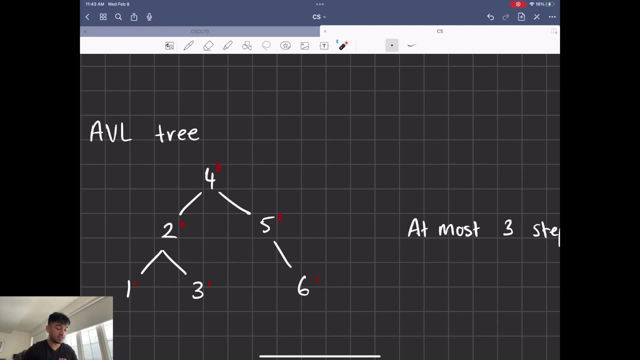 then same thing with 4, it's going to be 3. And likewise on this side. So you see that you have at most 3 steps And with that height variable we can rotate it as we need. So, AVL trees, use a. 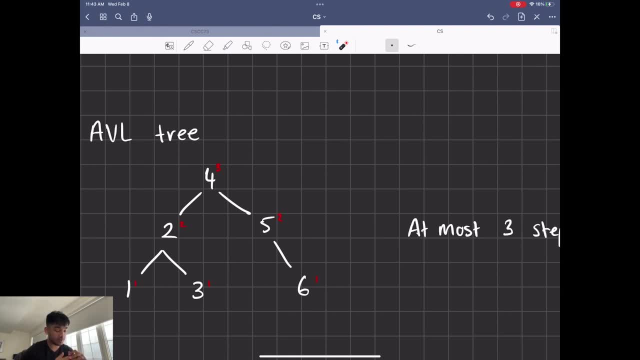 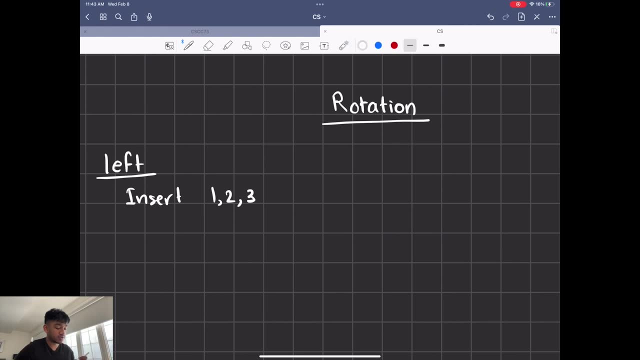 little bit more memory because they store the height, but it's a lot more efficient time-wise. So let's talk about how you would insert into an AVL tree using this rotation. So let's insert 1,, 2, then 3.. So it starts off just like a binary tree: You have 1, and then you have 2. here Let's. 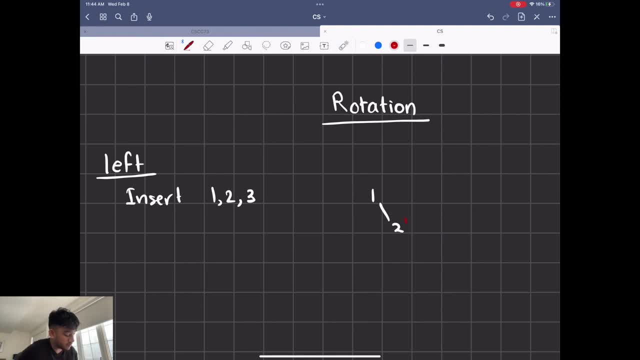 quickly draw out the height for each one. So this one's going to have a height of 1, and this one's going to have a height of 2.. Now, when you insert 3,, the heights are going to change to 1,, 2, and 3.. 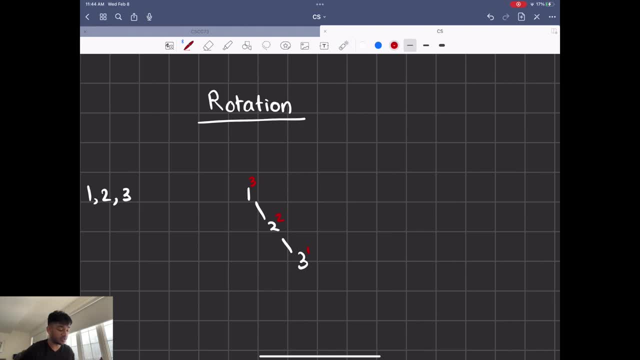 And this isn't optimal anymore, because once we insert 3, it's not balanced anymore, And the way we find out if it's balanced or not is by creating something called the balance factor. I'm going to call it BF for balance factor, and it's going to be the height of the right subtree minus the height. 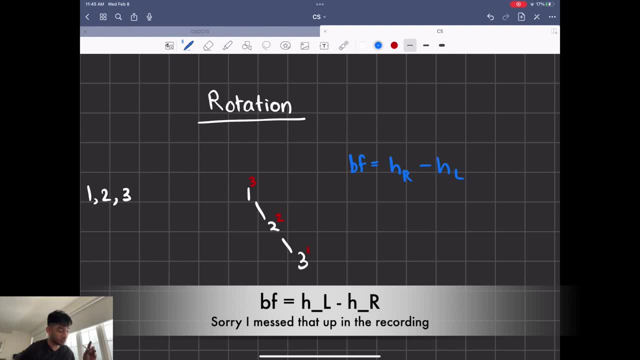 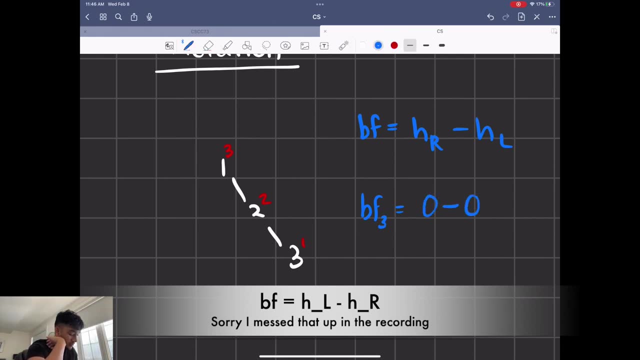 of the left subtree. I'm going to label it blue just so that we're not confused with the red. So let's find the balance factor of node 3.. It's going to be equal to 0 minus 0, because the heights of the subtrees 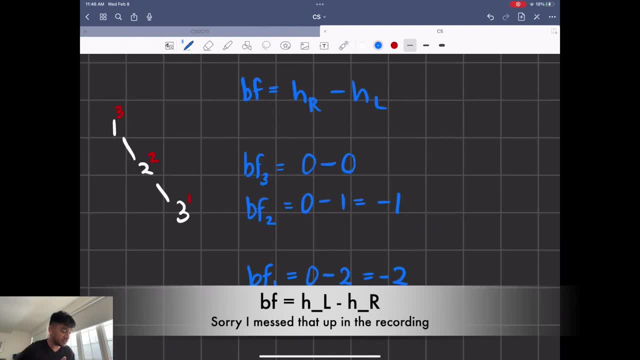 for the left and right are 0, because they're not there. The way we keep it balanced using these balance factors is by making sure that no balance factor is greater than 1 or less than minus 1.. So in this case it's okay. So the only acceptable values we have for BF is going to be: 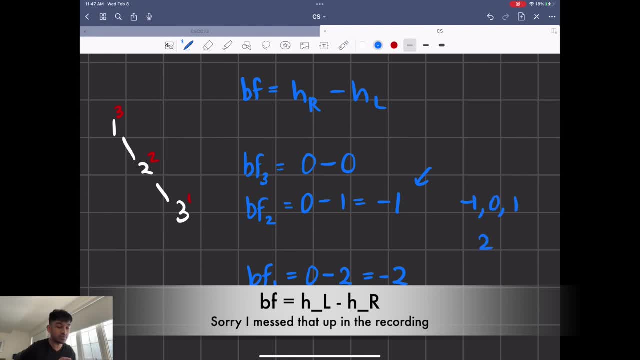 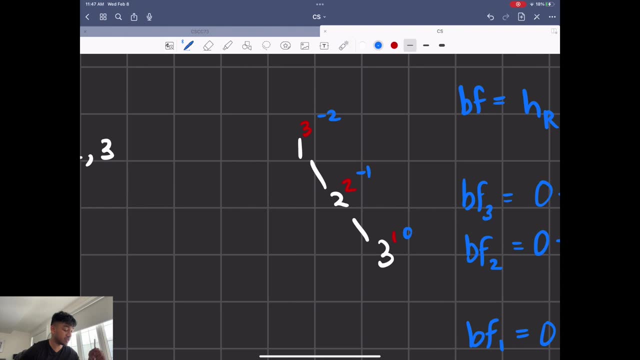 minus 1,, 0, and 1.. If it ever goes to 2,, we're going to have to balance again. So we're going to have to do something about this 1, because it has a balance factor of minus 2.. So what you do is you go to the next balance factor. 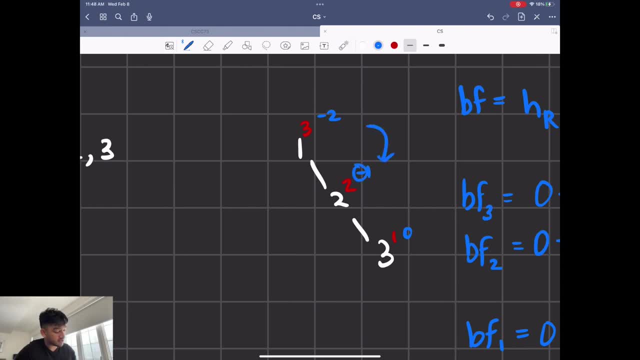 which is 2 here, and you're going to see that they're both the same sign of negative. So in this case we can do a left rotation. This means that we pivot on 2, and we make 2 the head. 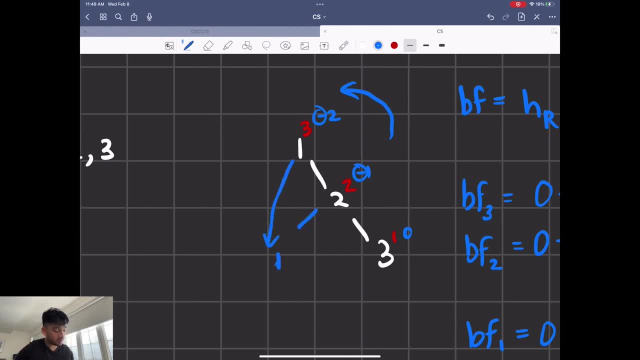 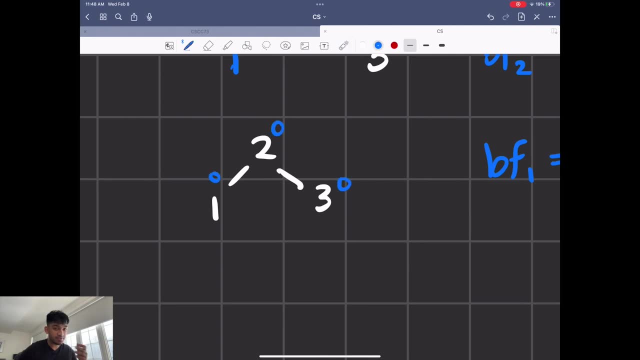 and we bring this down here as the child of 2.. So our new tree looks like this, and you can see that the balance factors for these are all between minus 1 and 1. In fact, they're all 0,, so it's. 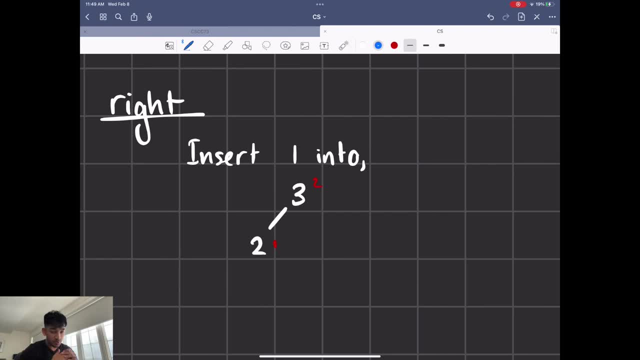 perfect. So that was left rotation. Let's talk about right rotation real quick. We have this AVL tree and we have 3 and 2, and we have the heights of them, So we have 1.. We're going to insert it just. 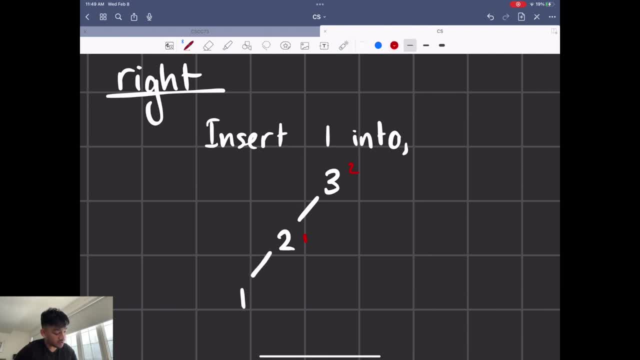 like a regular binary tree. We're going to have 1 here. We're going to update those heights, So it's going to be 1,, 2, 3.. Now, if you look at the balance factors, you can pause the video if you. 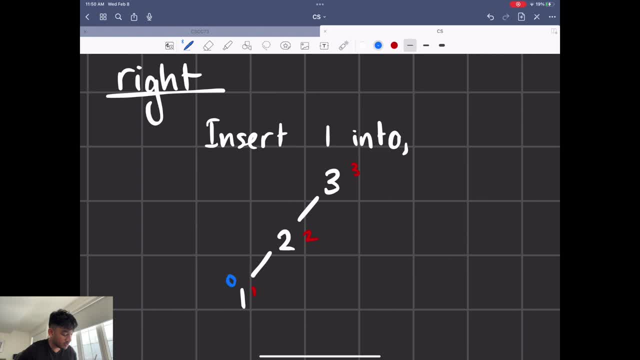 want. but let me do them real quick. This one is going to be 0.. This one is going to be positive 1, because it's a right child, And this one is going to be 2, because there's a right tree of. 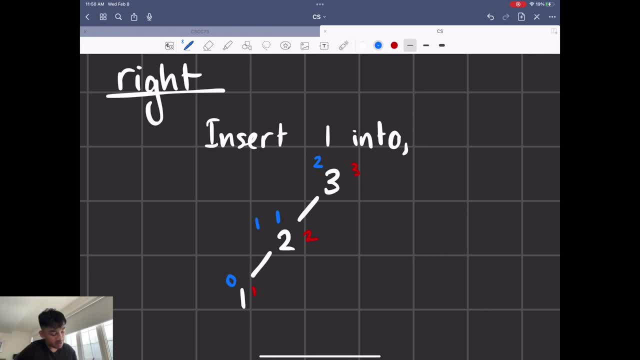 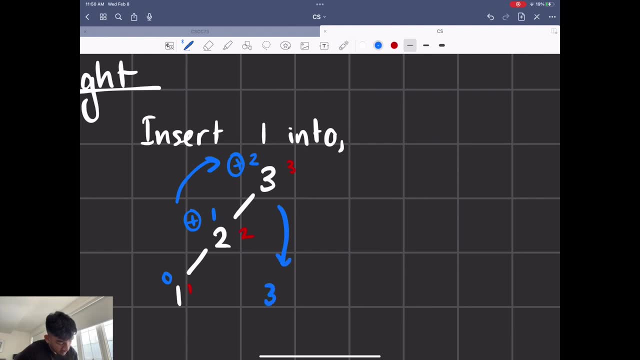 height 2.. 3 is 0, because there's nothing there. Now, like you see again, they're both the same side. So what you do is you just do a right rotation. So 3 would come down now here and 2 is going to. 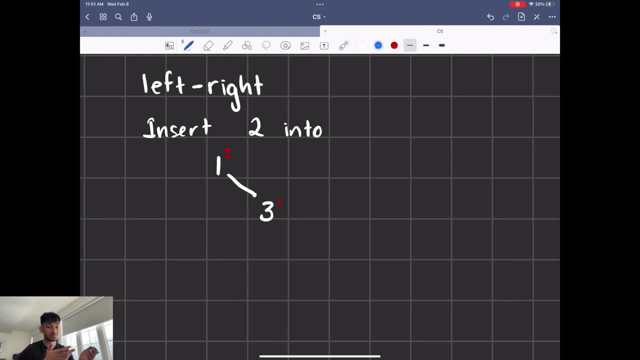 be your new parent, And so this is what you're going to have. Seems pretty simple so far. Let's talk about some complex rotations. So let's talk about the left-right rotation. Now, if we wanted to insert 2 into this new binary tree of 1,, 3, it's going to be same as a binary tree. We're. 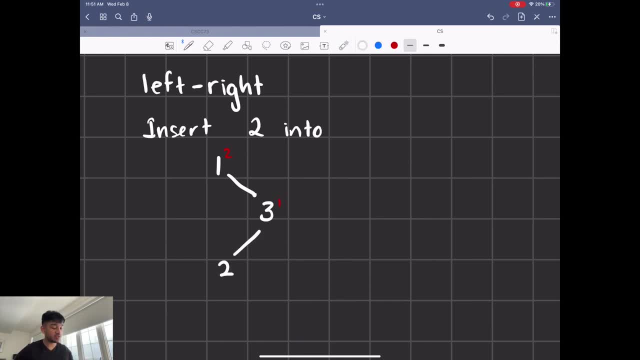 going to traverse down this and we're going to see that 2 comes here. So, as you can see, it's not really a linked list, because it doesn't follow this path anymore of this or this. Right now. it follows this path of this weird shape And you're going to. 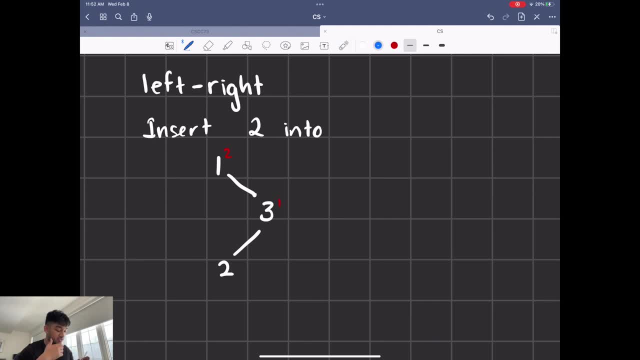 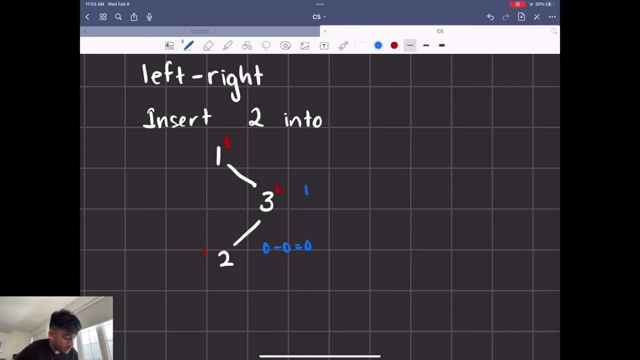 see that the balance factors actually are different for these cases. Now, if we find the balance factor of each of these, it's going to be 0 minus 0 to 0.. In this case, you're going to take 1 minus. 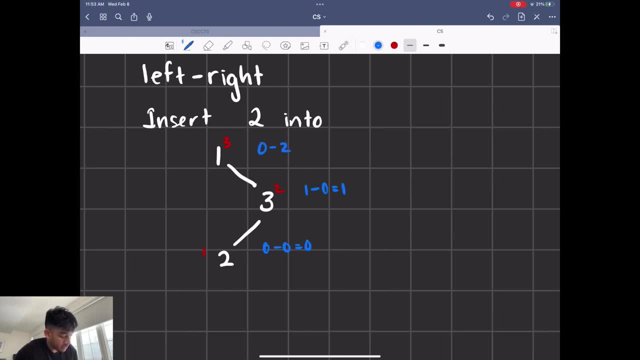 0 is equal to 1.. In this case, you're going to have 0 minus 2. And the 2 is what you get from here, And this is going to be minus 2.. So you're going to see that the top one has a negative balance. 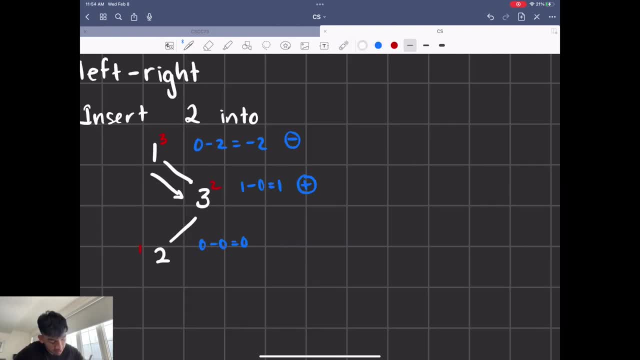 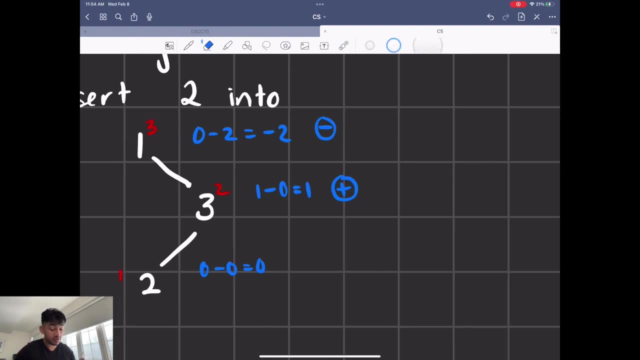 factor and this one has a positive balance factor. So we can't really rotate these two anymore because they have opposite signs And if you think about it, you can't really visualize rotating this. Not really. So in order to do that first, 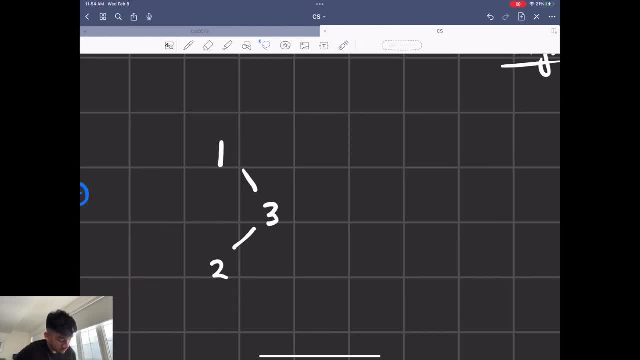 what we need to do is make it a straight line by rotating these two, So you're going to see it as 3 coming down and 2 coming up, And then you put the line here And now you have this new binary tree where you have the same sign again, And we've seen this before. It was in. 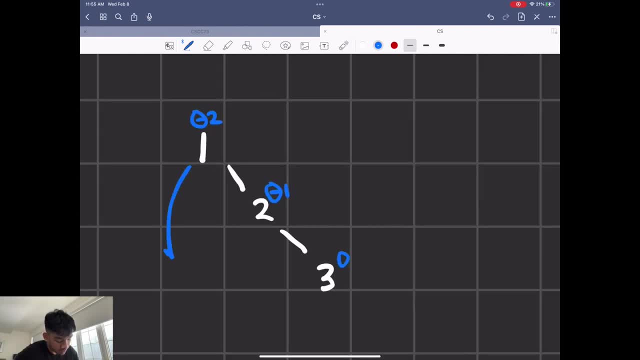 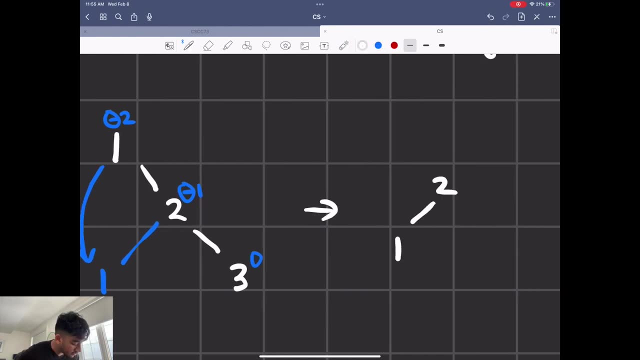 the left rotation that we did. So all we're going to do is rotate this 1, bring it down here and we're going to add it here. So our new tree is going to be 2,, 1, 3.. That's pretty much it Let's talk about. 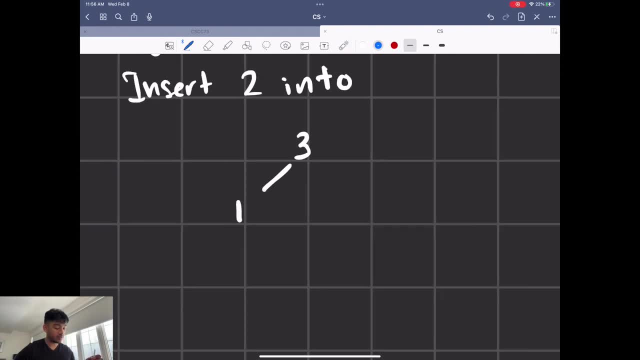 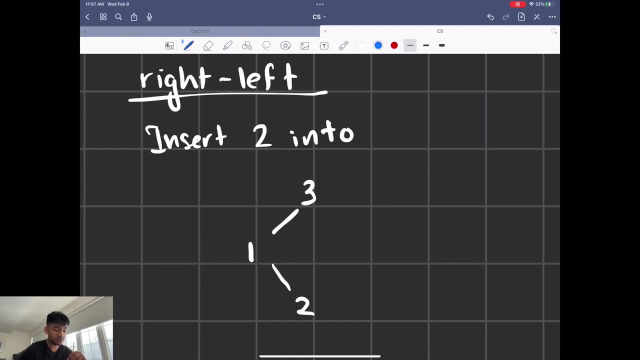 right-left rotation. That's the last one. So now you're going to have 1 and 3, and you're going to want to insert 2.. So right-left rotation looks a little bit like this: Let's insert 2 here. I'm not going to be writing the heights anymore for every single one. 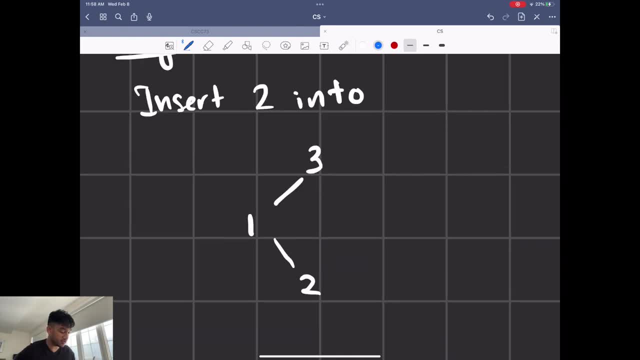 but let's talk about the balance factor. So the new balance factors are going to be 0, minus 1, and then positive 2.. So we have to balance because there's a 2 here and these 2 are opposite signs again, so we can't really rotate it anymore. 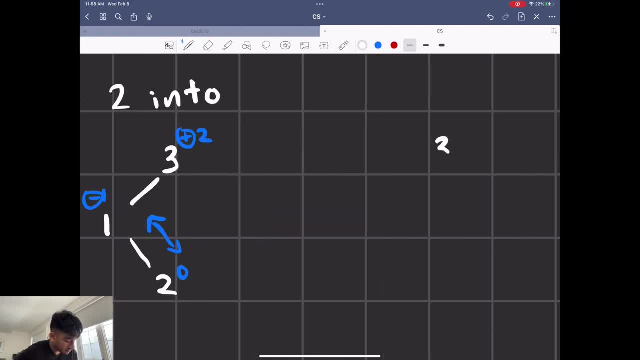 So what we do is we swap these two again. So now we're going to have 3,, 2, and then 1 here. So the balance factors are going to be 0,, 1, and 2. And they're both the same sign. 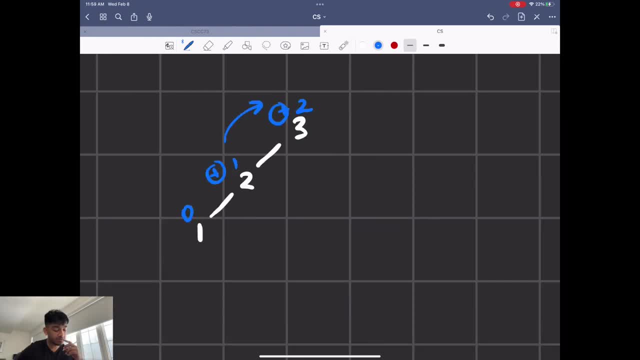 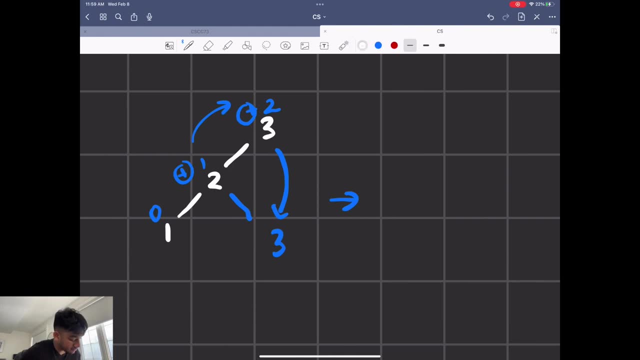 so you can rotate it, And you can actually rotate it right, just like how we did before. So we're going to bring 3 down here, like that. So our new graph is going to look like: 1,, 2, One, two, three. 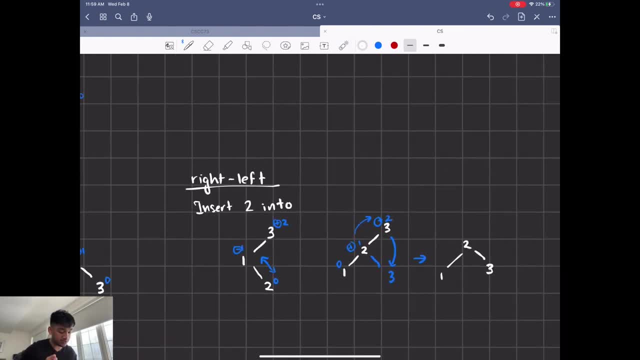 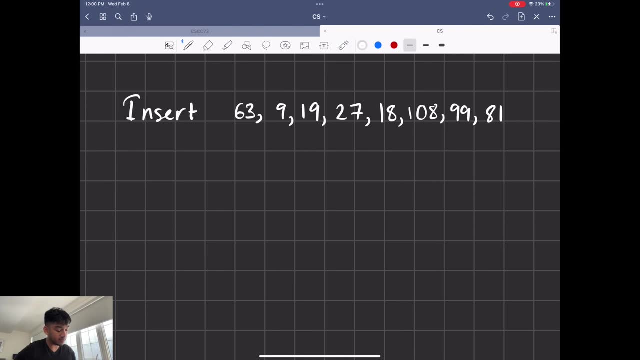 And just like that it's balanced, And we use all these cases whenever we insert something. Let's use this example I saw on the JavaPoint website. I'll have the link in the description if you want to check that out too. So let's insert it just like a regular binary tree. 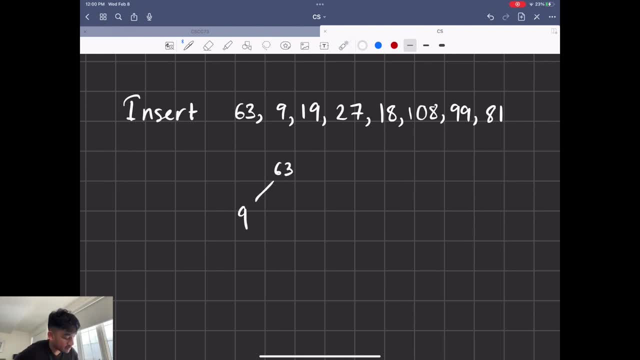 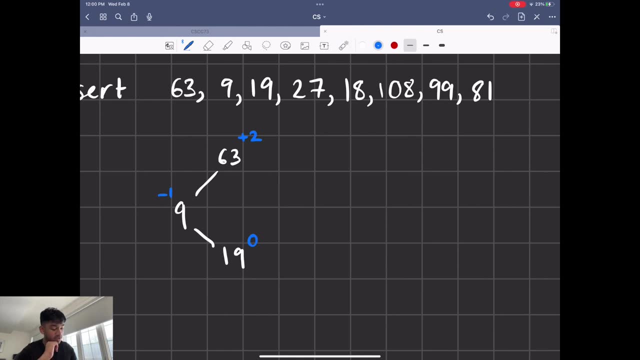 So we're going to have 63.. 9 is going to come to the left, And then we have 19 come here And if we draw the balance factors already they're not balanced anymore. So let's do a left-right rotation in this case, because they have opposite signs. 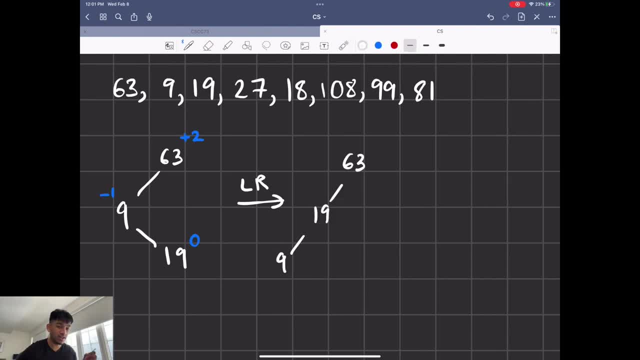 So we switch 19 and 9 first, And now we're going to rotate that. So we swap 9 and 19.. And now we're going to rotate it to make 19 the top. So we're going to rotate and bring 63 down here and bring the root here and then get rid of that. 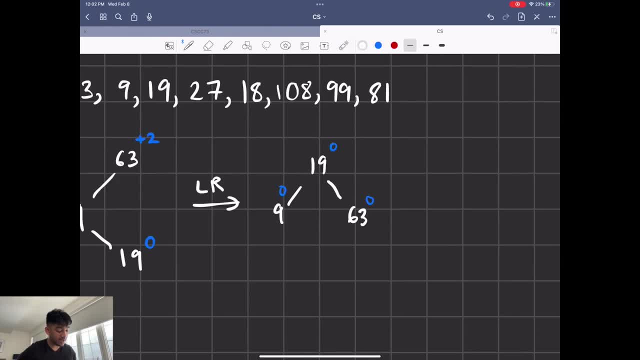 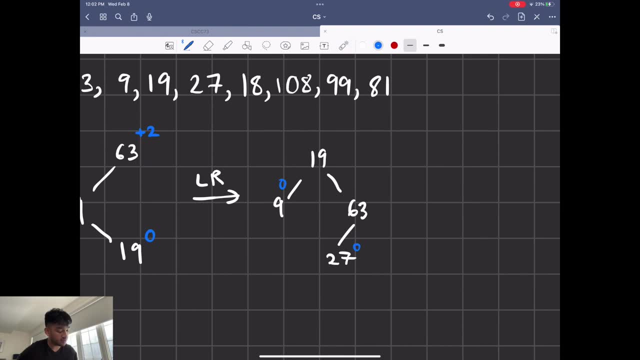 So this is our new tree And you can see it's balanced. Let's now add 27.. 27 would come here, So the balance factor would change on the right side. Now, this is going to be 0.. This one is going to be 1.. 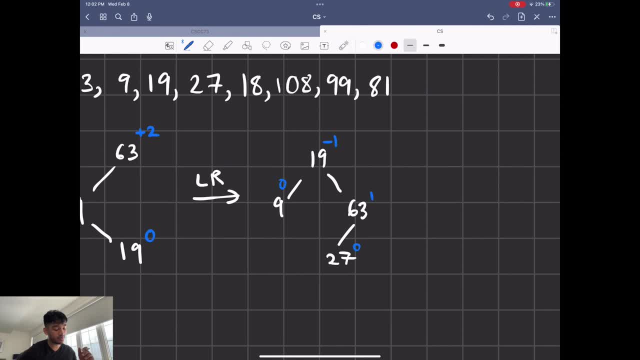 And this is going to be minus 1.. So we're in between 1. And negative 1.. So we're good, Let's add 18.. 18 would come here And we're going to update the balances accordingly. So this is going to be 0.. 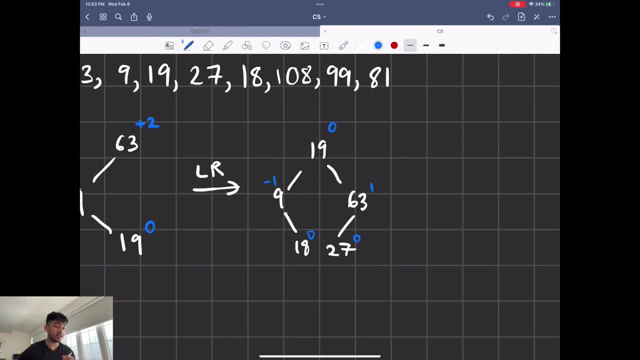 This one is going to be minus 1.. And this is going to be 0 now, because both left and right subtree have a height of 2.. Let's add 108 here, It's going to have a balance factor of 0.. 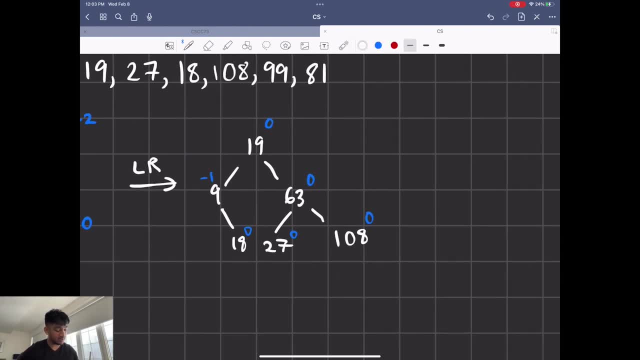 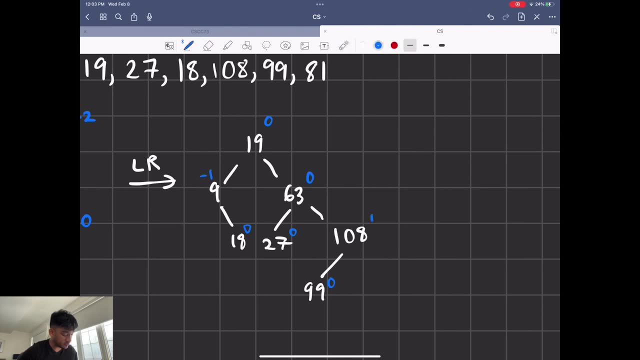 This is also going to be 0 now. And now let's add 99.. 99 would come over here. Balance factor would be 0. And this would be changed to 1.. This would be changed, And this would be changed to minus 1.. 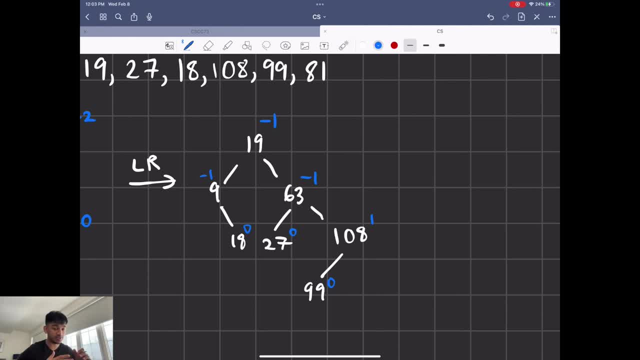 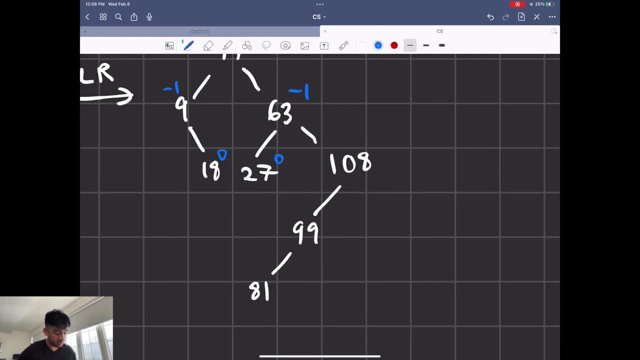 And so would this. If I'm going too fast, feel free to pause it and then check it out yourself. Finally, let's add 81 here, So 81 is going to be right here, And let's test the balance factors again. 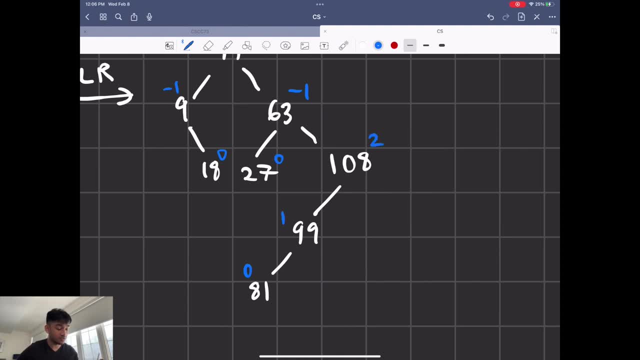 So this is going to be 0.. This is going to be 1. And this is going to be 2.. So we can't have 2.. So we're going to have to rotate it again, And you know it's going to be a right rotation, because we have the same signs here. 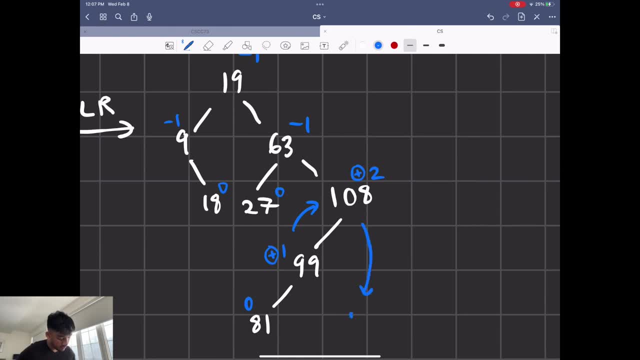 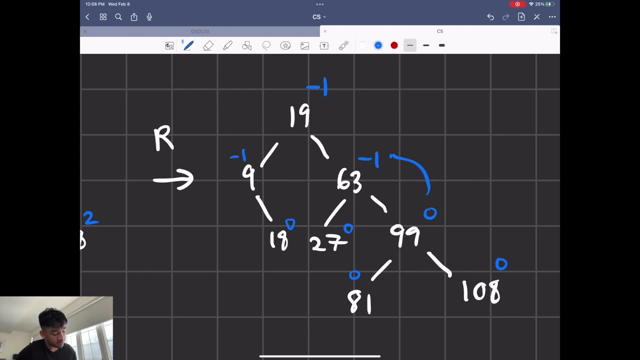 So yeah, let's rotate. So 108 would come down here now. So now these are balanced and everything else, say, is pretty much the same. So this is going to be minus 1.. And then this is also going to be minus 1 still. 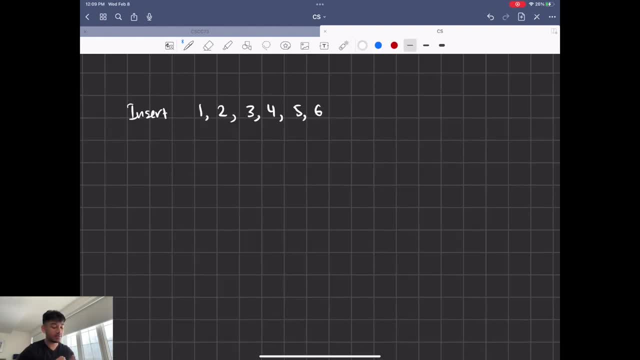 So that's how you get a balanced AVL tree by inserting these values. Let's talk about inserting these values, Like we saw that this would give us a link list when we try to insert into a binary tree, And let's talk about how we would do it with an AVL tree. 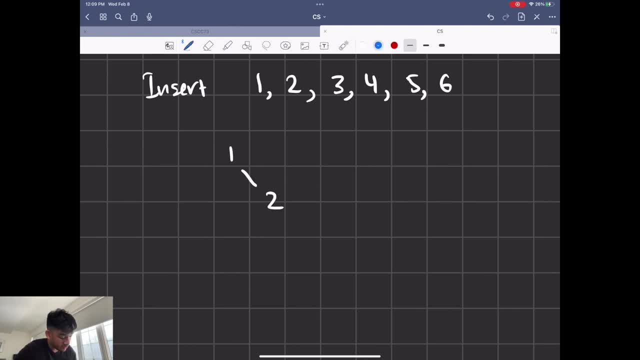 So we start off with 1, 2.. Balance factors are going to be 0 and negative 1 here. When we add 3, this is going to be 0. This is going to be negative 1.. And then this is going to be negative 2.. 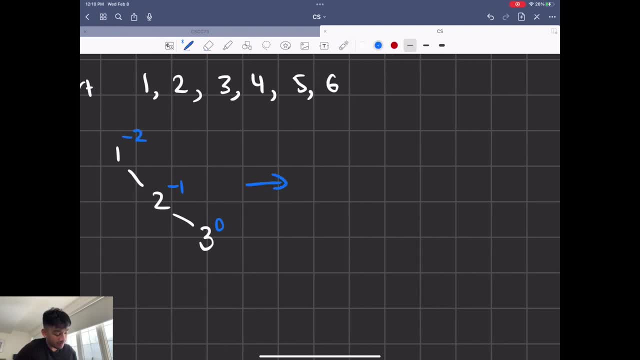 Like that. you have to make a left rotation, So 1 would come down here And then 2 would be the root. So our new thing is going to be 2, 1, 3.. Let's insert 4 then. 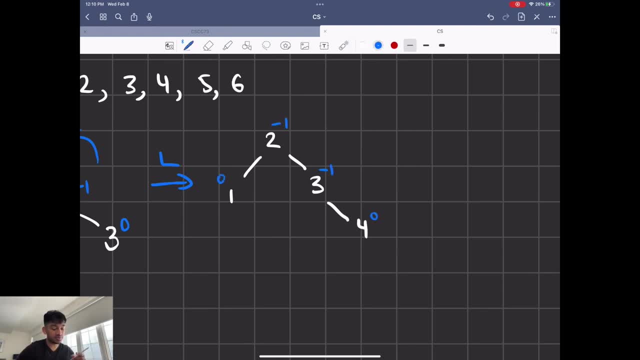 4 would come here And you're going to get these balance factors so we can keep inserting. So let's add 5. And the balance factors are going to be 0, minus 1, and minus 2.. So we're going to have to do a right rotation. 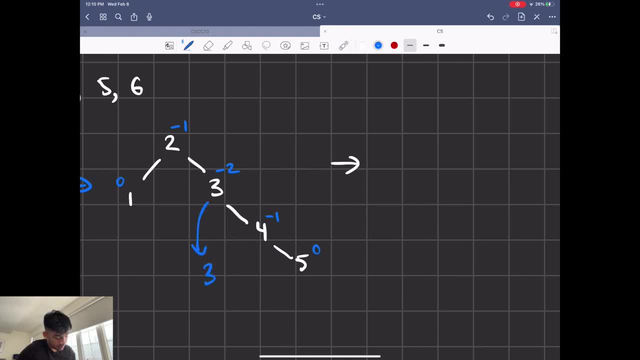 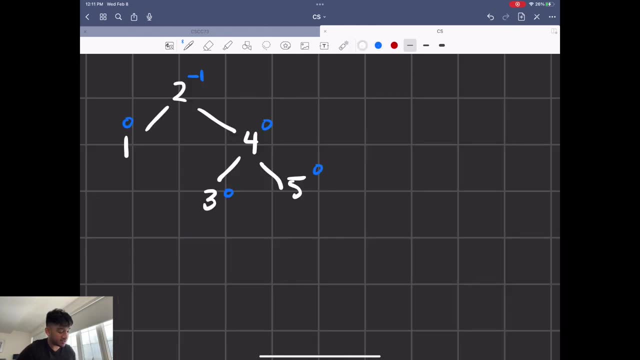 On this pivot. So we bring 3 down here, Connect it to 4. And make 4 the root of the right subchild of 2.. So this is what we're left with, And let's add 6 finally. So we add 6 here. 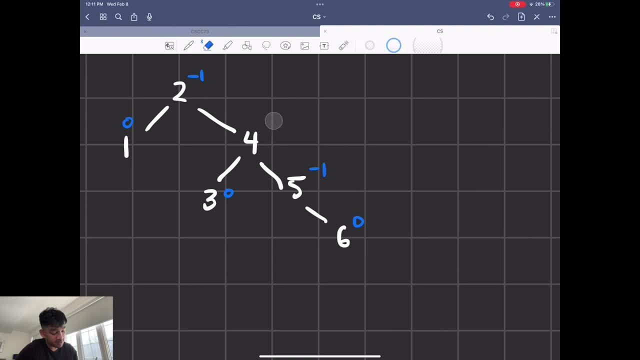 This is going to have a balance factor of 0. This one is going to have negative 1.. It's also going to have negative 1. But when you look at this one, it's going to be negative 2. Because this has a height of 1.. 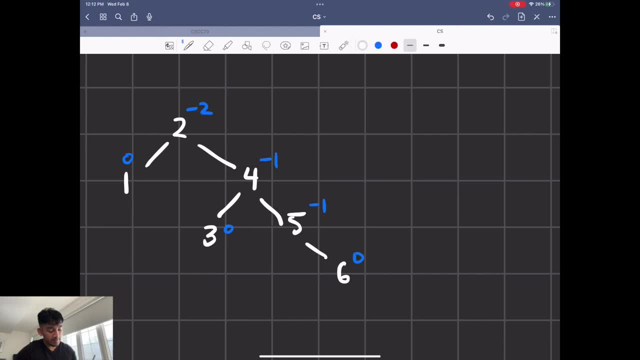 And then this has a height of 3.. So 1 minus 3 is minus 2. And you can see that this and this have the same sign. So it's just going to be a left rotation, But it's a little confusing now. 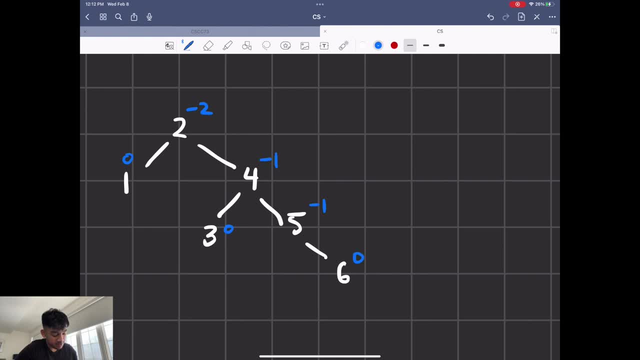 Because we can't really do that with this value right here. So we can't exactly just rotate 2 down here, 2 and 1. Because 3 is right here. So what you do is Just forget about that 3 for now. 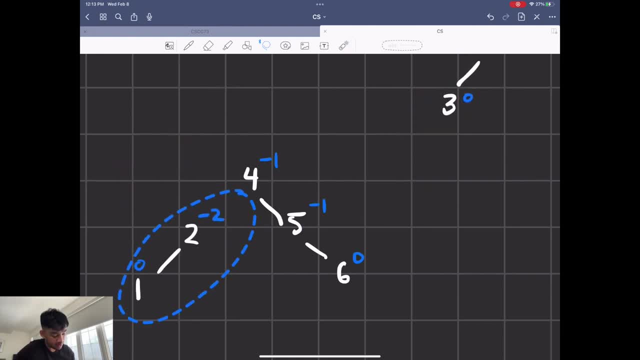 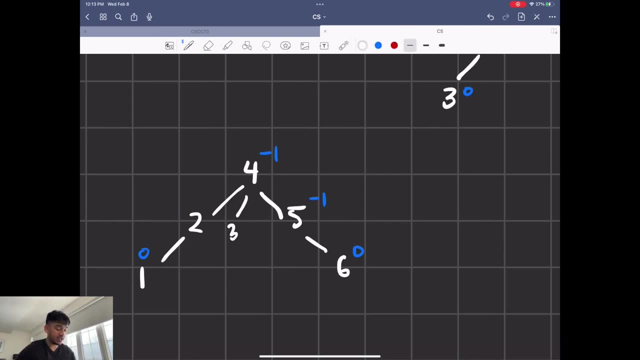 Just take that somewhere else. You bring that 2 down here, Just like you did before, And that 3 that we initially had over here We're going to have 4, because it's less than 4.. But it's also greater than 2.. 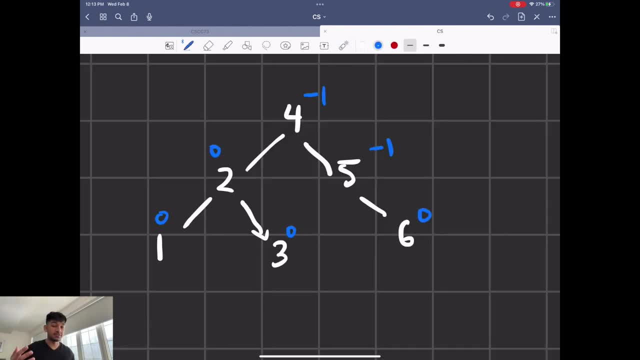 So what we're going to do is we're going to add 3 here now And all it's done is balance again, And that's what we had before. So this is going to take at most 3 steps to traverse through. Let's talk about deletion real quick. 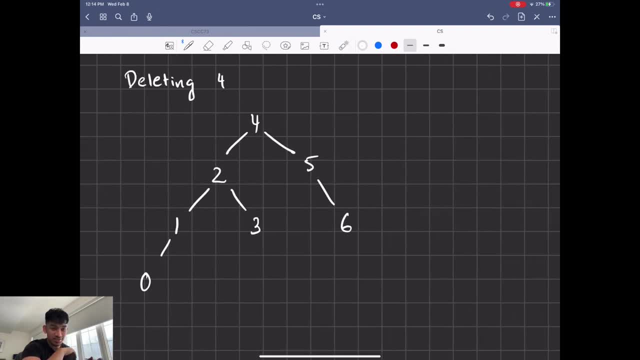 It should be very simple. It's just like deleting for a binary tree And then just balancing it again, And balancing is just rotating. So let's do that. So if we delete 4, we're going to take the rightmost value of the left subtree. 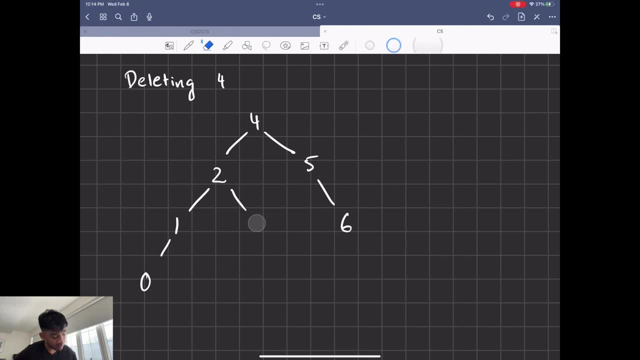 So it's going to be 3 right here, We're going to add 3 to the top here, And then the first affected parent node is going to be 2.. So let's look at the balance factor of 2.. So the balance factor of 2 is already minus 2, which we can't have.